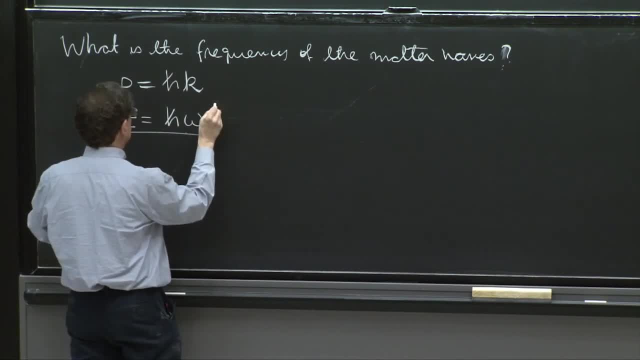 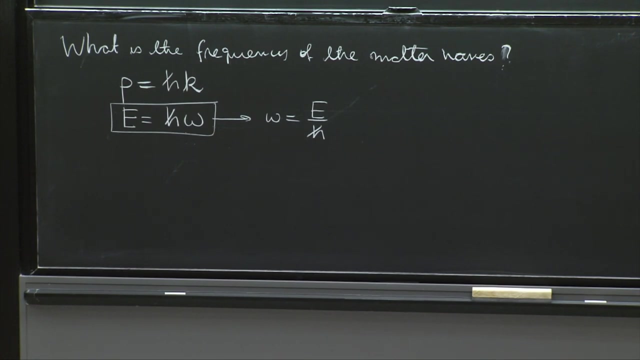 So the frequency. So this equation is the one that now completes the story. Omega is equal to E over h bar, And the wave replaces omega by omega in terms of the energy, Fixes omega in terms of the energy, And we're going to say a few things. 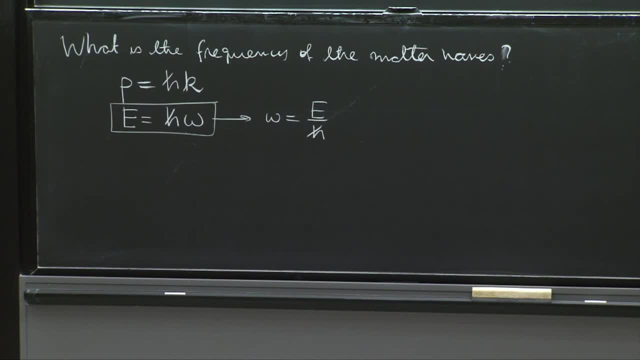 In fact, this will be an interesting digression into an important subject about waves. that illustrates why this answer makes a lot of sense And that's really all you can do at this moment- that you do this thing and with this you get quantum mechanics. 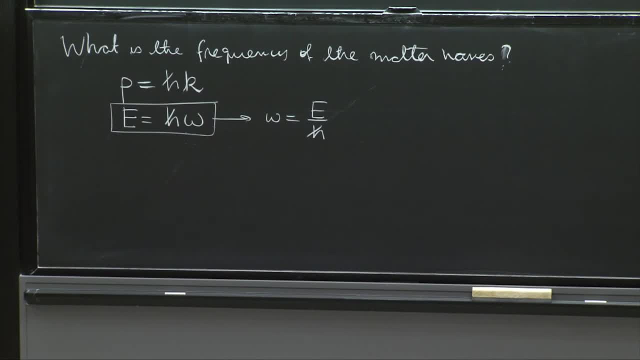 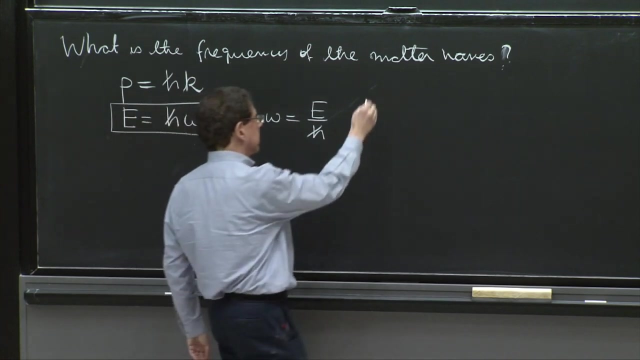 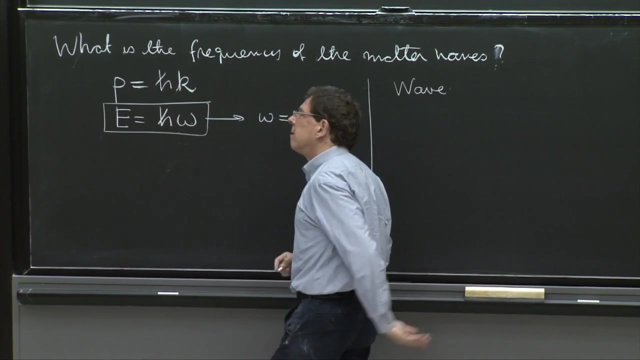 So the best thing we can do is explain why it makes sense in a number of ways and then hope that the theory that you build makes full sense. So I want to remind you about velocities of waves. So if you have a wave now that has k and omega, 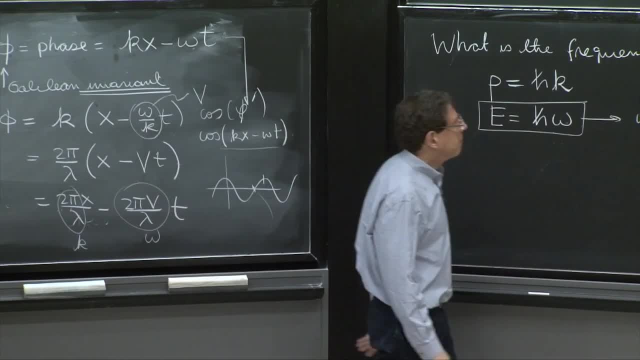 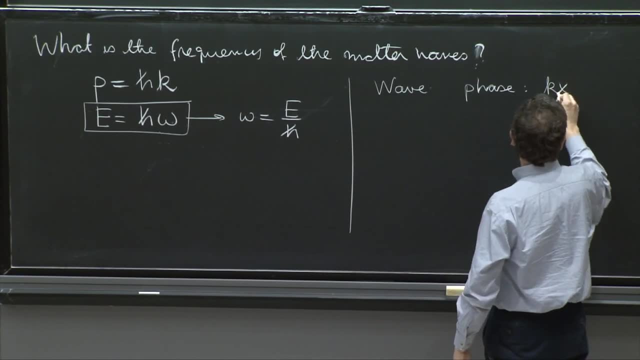 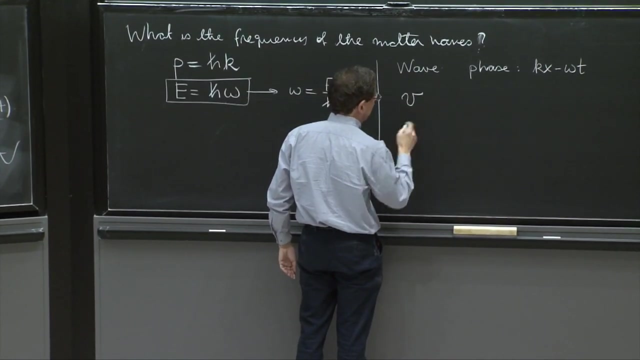 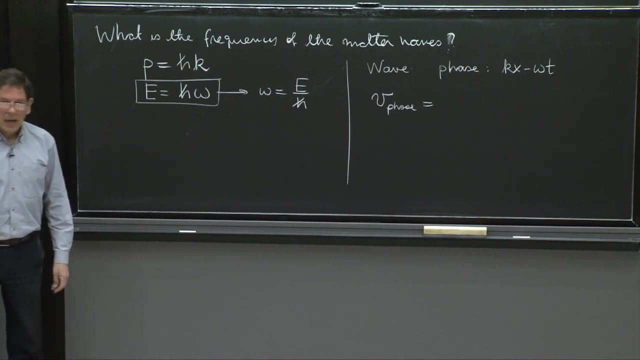 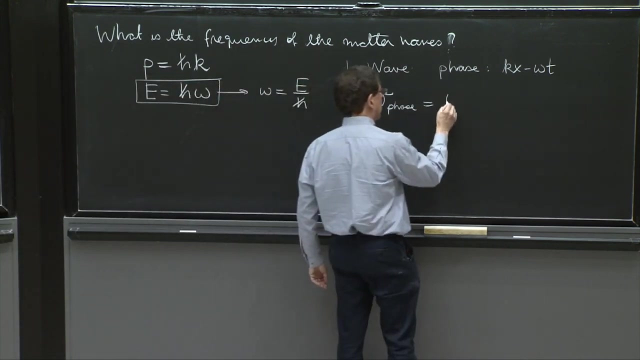 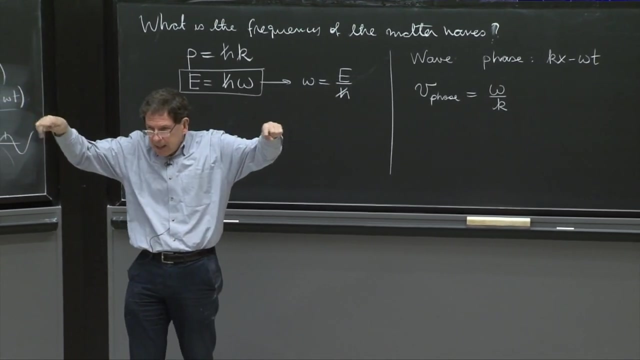 you have this thing: k minus omega wave with a phase kx minus omega t. Then there is something called the phase velocity and it's given by omega over k. It's the velocity in which the nodes and maxima of this plane wave move. 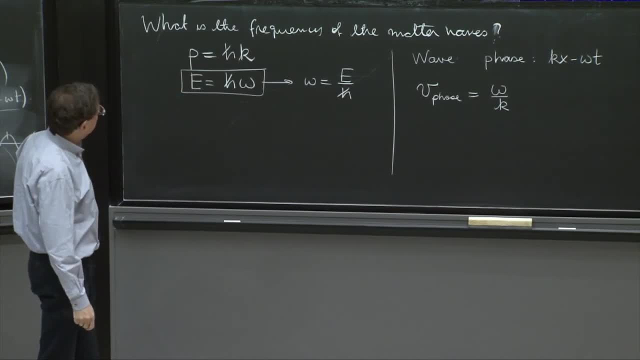 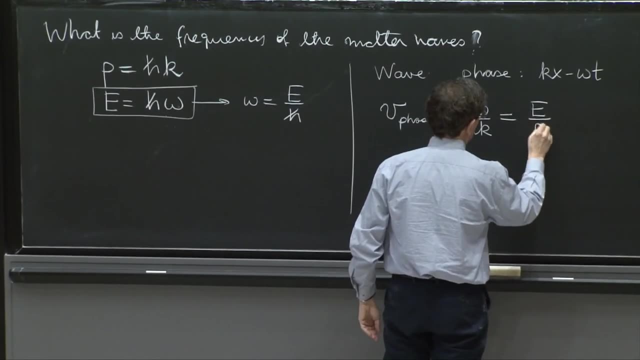 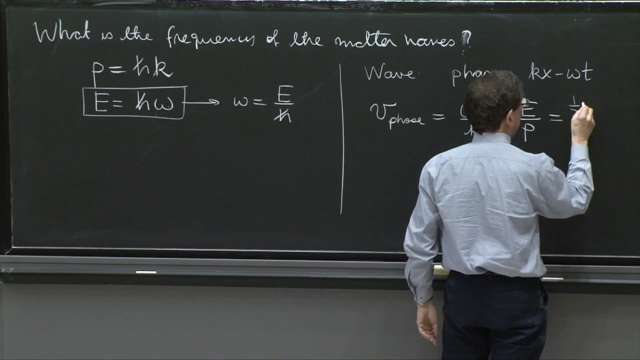 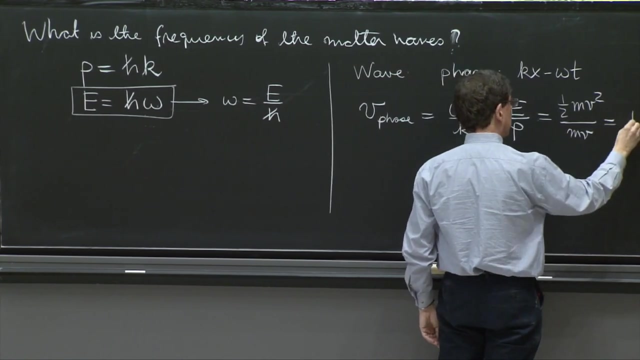 So let's see if this makes some sense. Omega over k is the same thing as e over p. We're non-relativistic, so let's continue. 1 half mv squared over mv, And this seems a little strange. 1 half v. 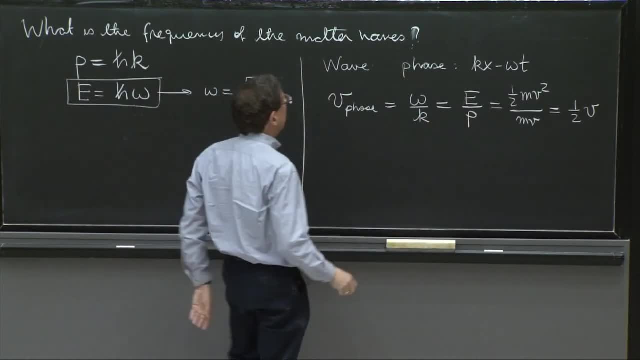 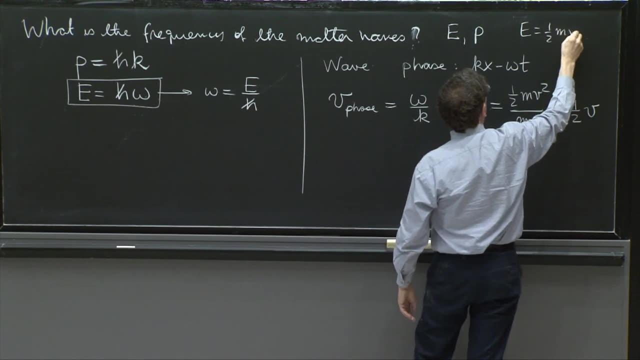 So if I have a particle- you see, this is matter- waves of energy, e and momentum, p And e is 1 half mv squared. The velocity of the particle, p is equal to mv. And now somehow, Somehow, Somehow. 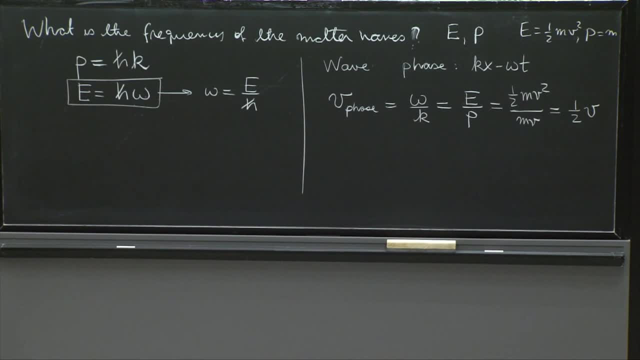 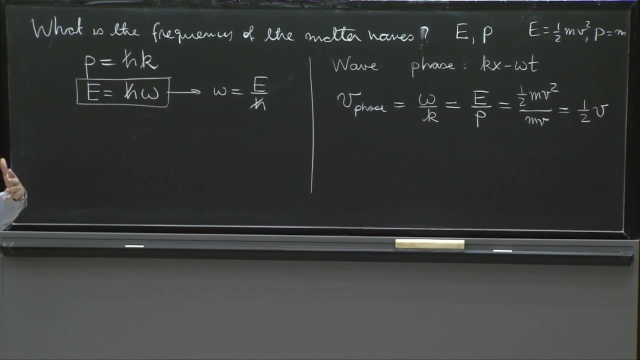 This wave seems to be moving with half the speed of the particle, And that looks pretty bad. What's going on? Well, this is the usual story with waves: If the wave itself doesn't a wave, a plane wave carries no real information. 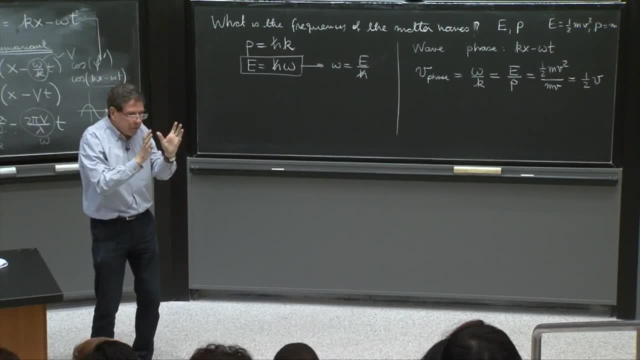 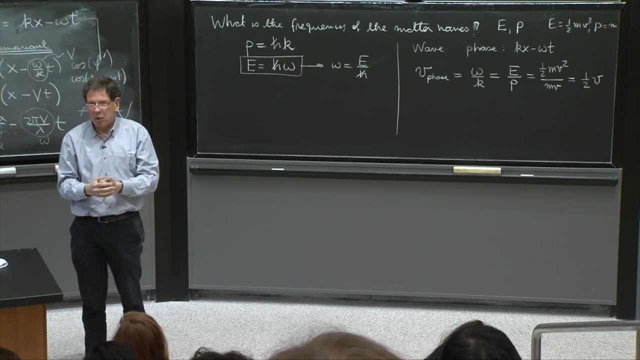 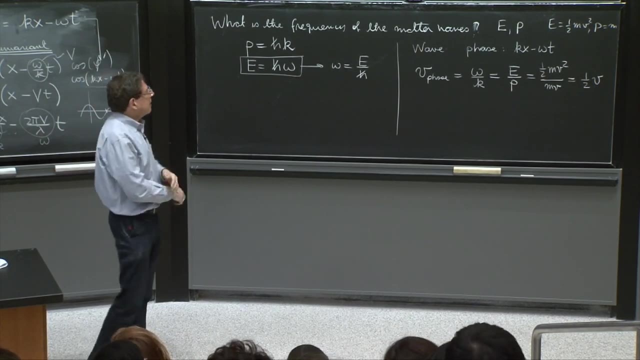 It's not the signal. So many times when you try to represent the particle or a little bit of information traveling, representing it with a plane wave is actually quite wrong. You have to represent it with a wave packet And therefore this phase wave velocity. 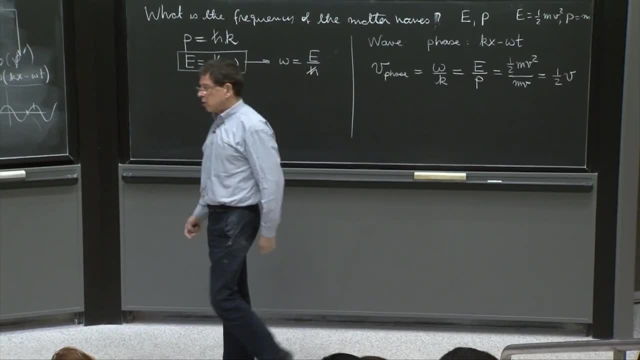 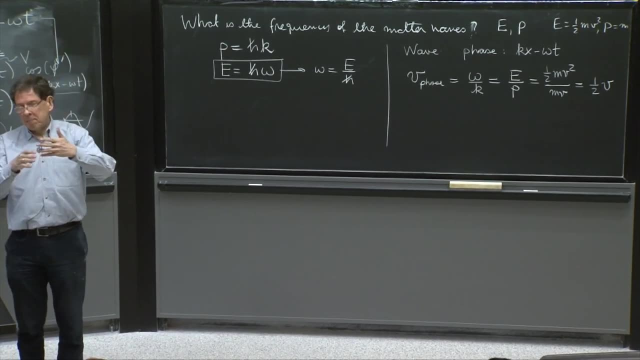 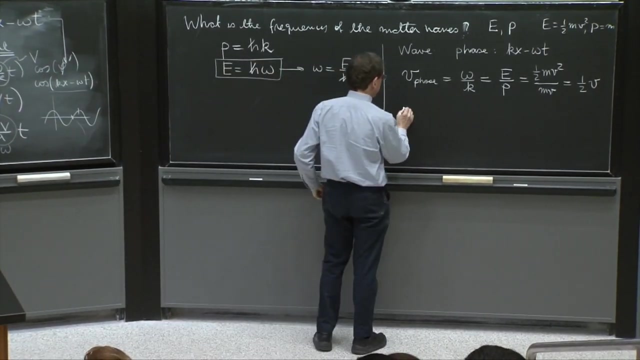 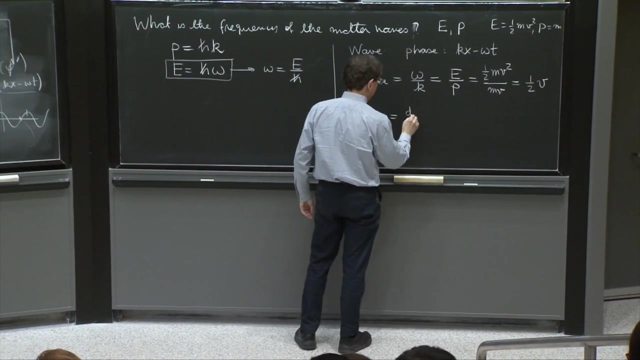 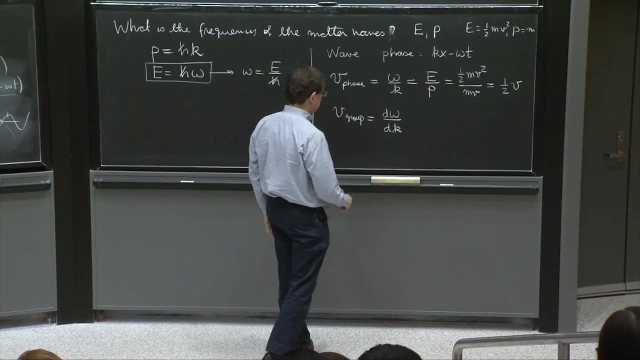 being 1 half of the velocity of the particle seems to just confirm the idea that first, these waves are a little strange And second, phase velocity is not very meaningful physically. The velocity that is more meaningful is v group velocity, And it's d, omega, dk, evaluated at the value k that you're using. 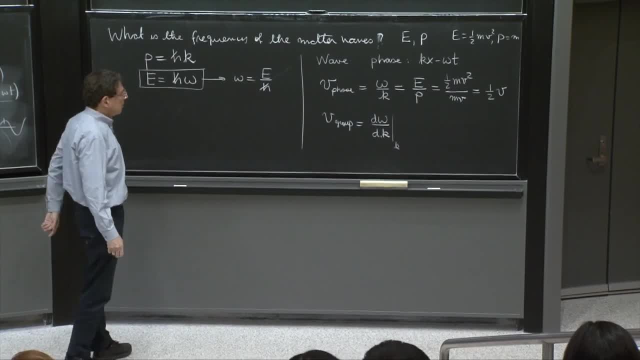 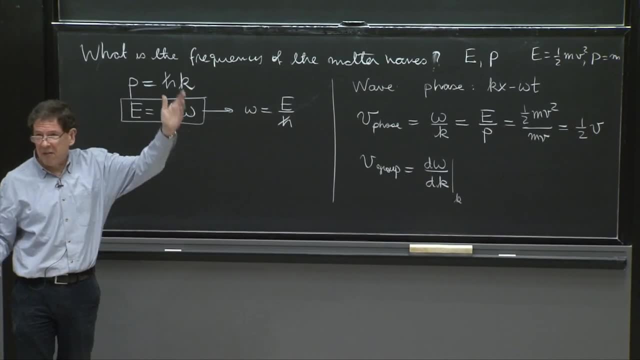 k is a proxy for momentum, So d omega dk may depend on k and omega. So if it's d omega dk, d omega dk is a function. Which value should you use? Well, the value at the k that you're propagating. 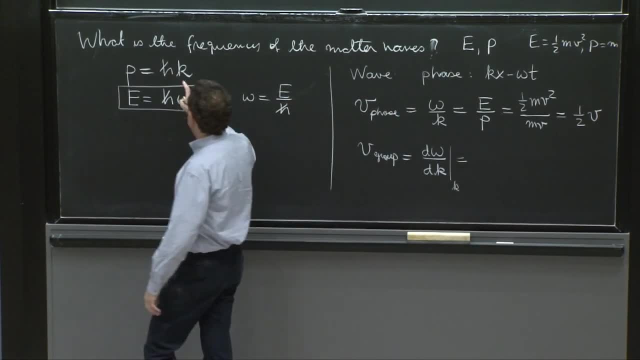 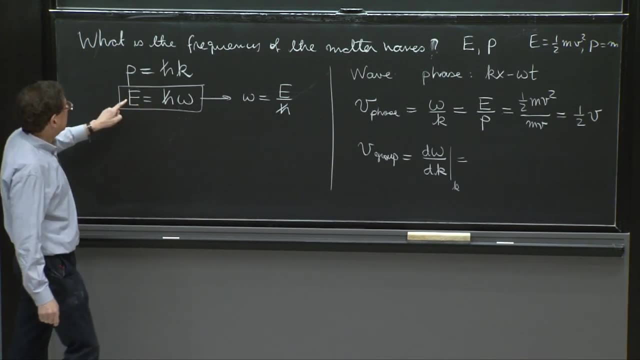 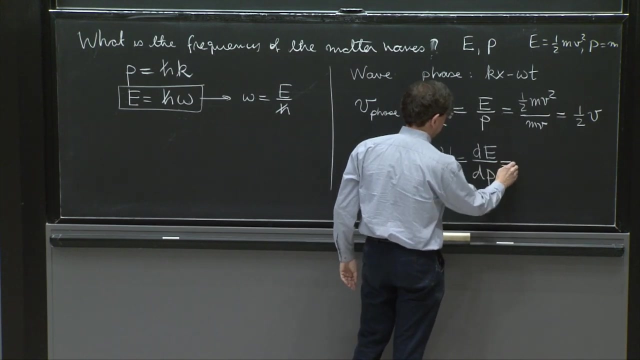 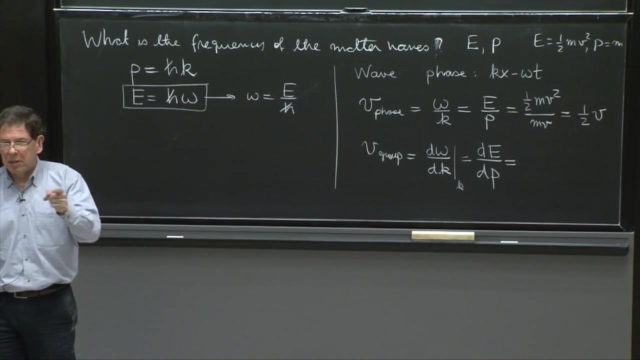 And this would be the same as d, omega. dk is, because of the constant separating, the same as d, e, dp. But what is the kinetic energy? Well, the kinetic energy in terms of the momentum. we wrote it last time, p squared over 2m. 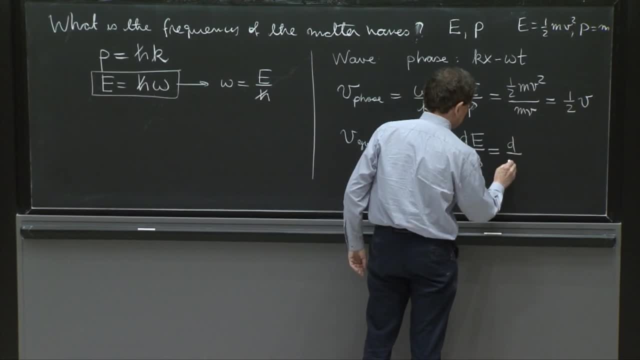 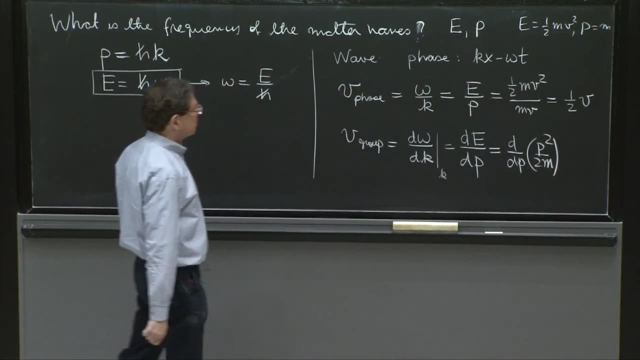 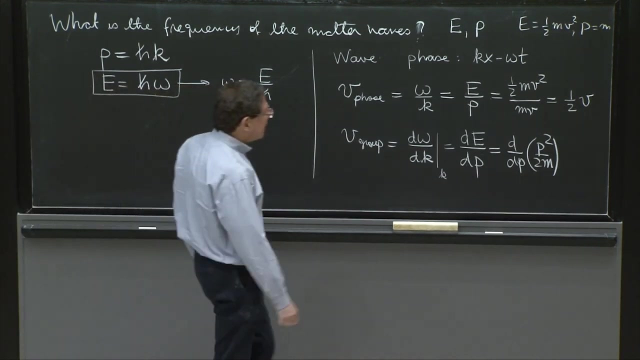 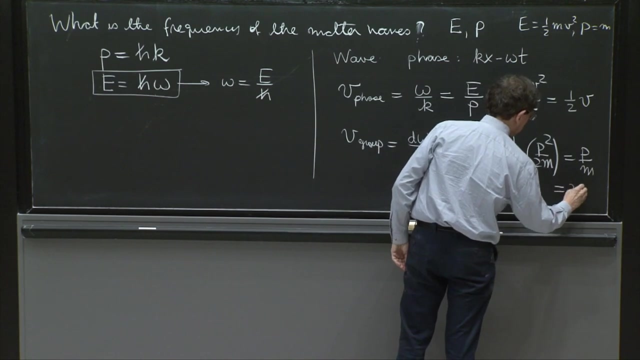 That's the kinetic energy expressed in terms of momentum. So this is d dp of p squared over 2m. Write p equal mv and you recover the kinetic energy. And this is just Because of the 2. p over m, which is the velocity of the particle. 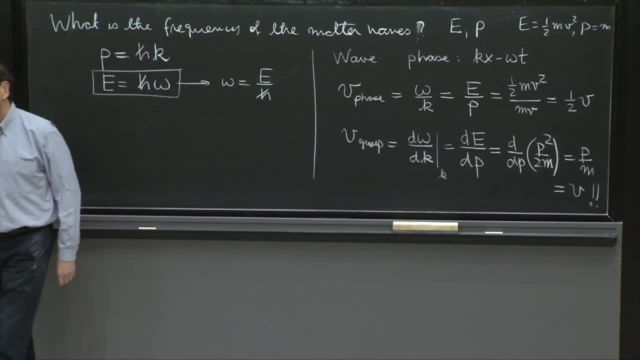 And this is the reason people believe de Broglie. De Broglie made sense because the group velocity of this packet would be correct, And that's a very beautiful result. Actually, it's true relativistically as well, If you put the energy and the momentum in relativity. 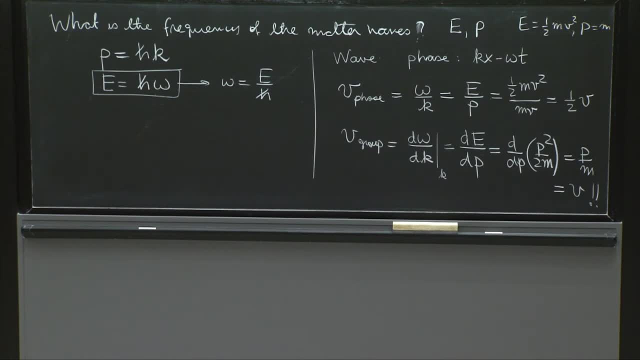 this answer comes out exactly the same, Perfectly well, So to a large degree, since it also works for energy and momentum in relativity. there was a motivation from relativity that I want to quote, although not elaborate on it too much. 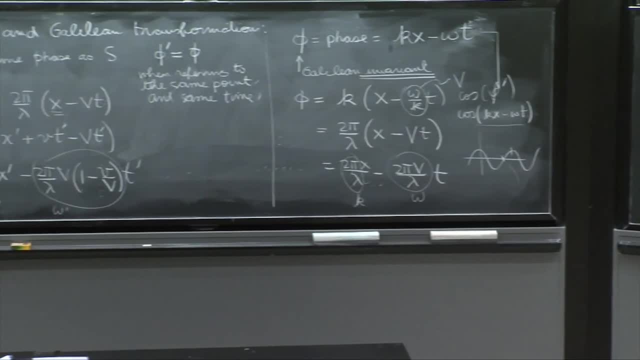 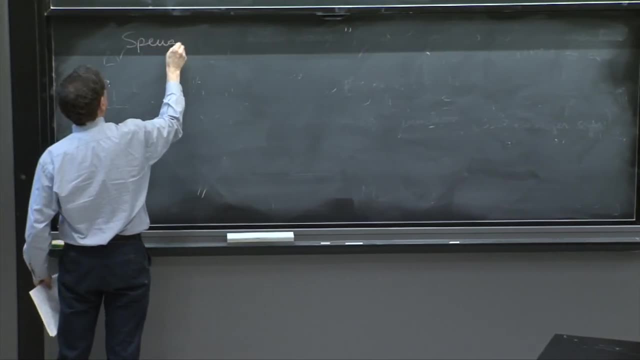 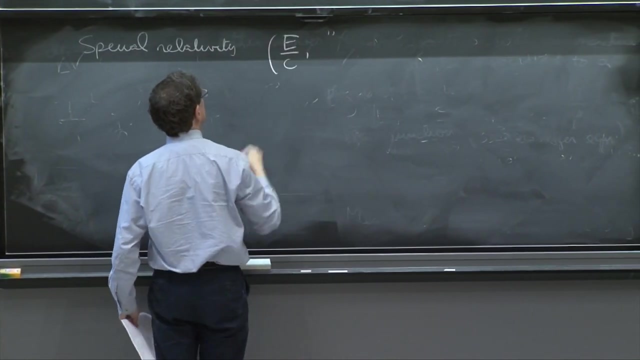 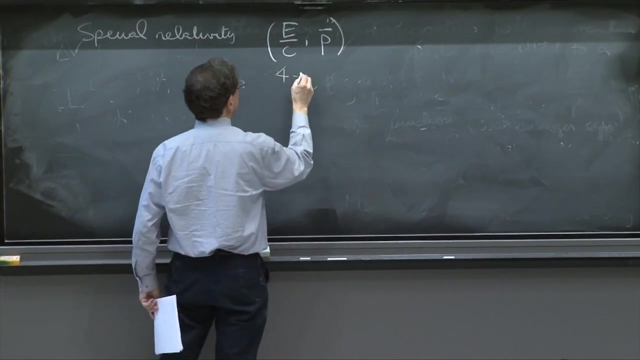 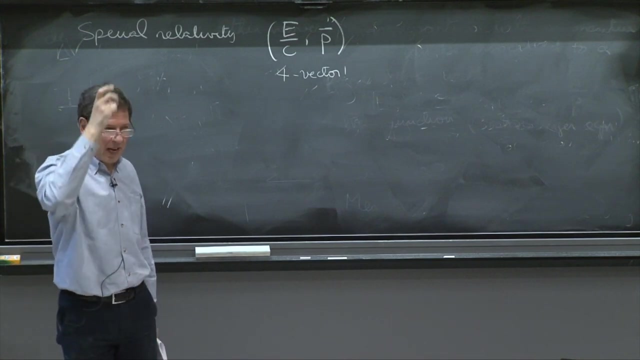 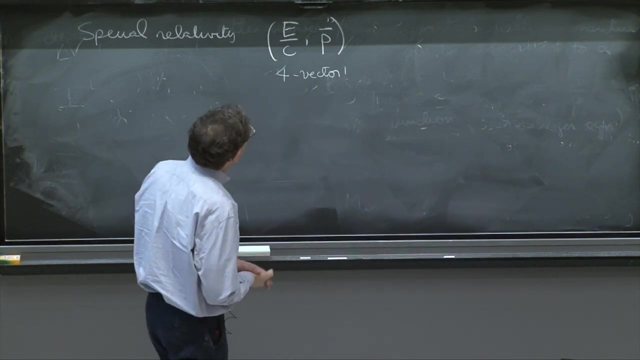 So the motivation Is that in special relativity the components of the energy divided by c and the momentum form a four vector, Just like position and time forms a four vector and it transforms nicely About with Lorentz transformation. e and p form a four vector. 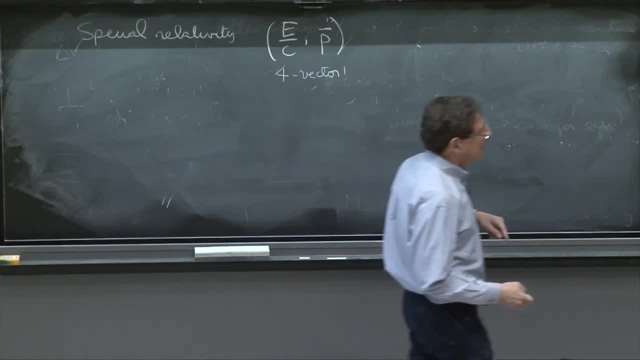 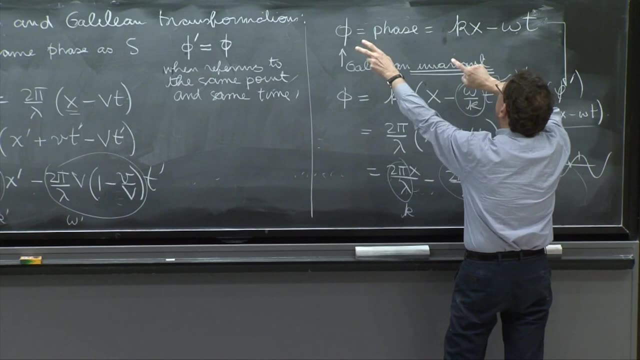 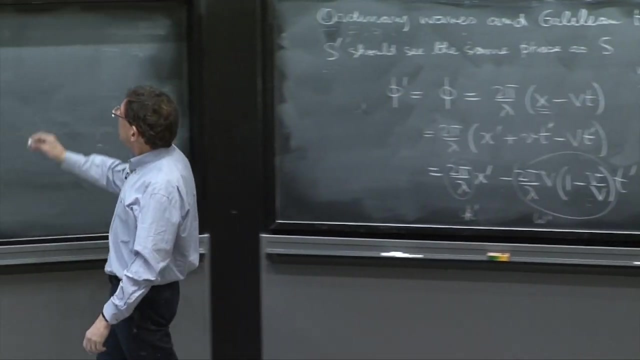 Nevertheless, when you consider phases like this and you have x and t that form a four vector, the good behavior of phases also imply that k and omega form a four vector. In fact, omega in relativity, omega over c and the k vector. 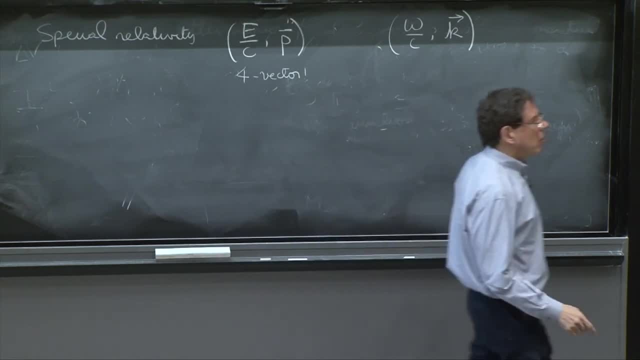 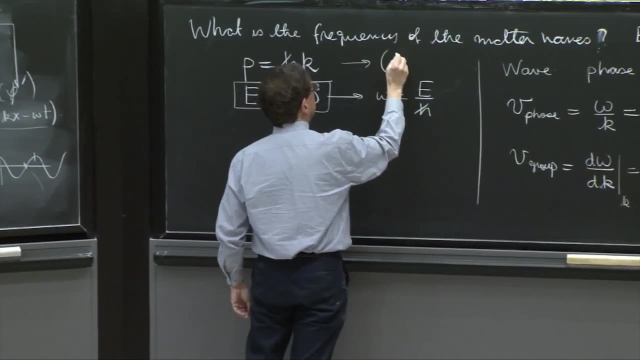 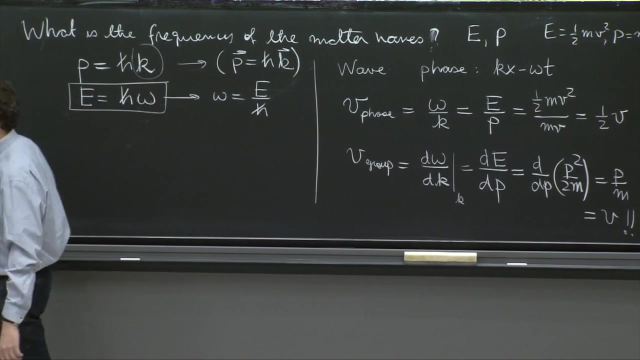 they form a four vector. You see in all the equations we've written and de Broglie. de Broglie, in three dimensions or more, really, is p vector equal h bar k vector, And k is usually used for the magnitude of this k vector. 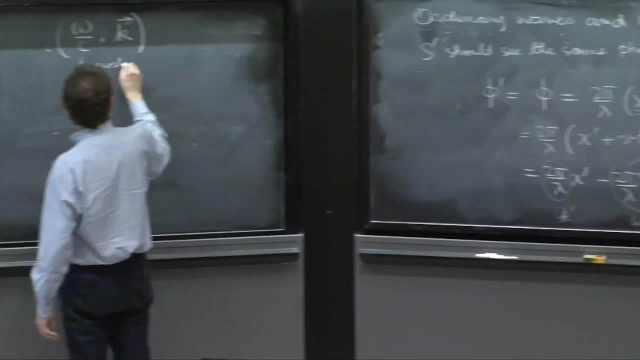 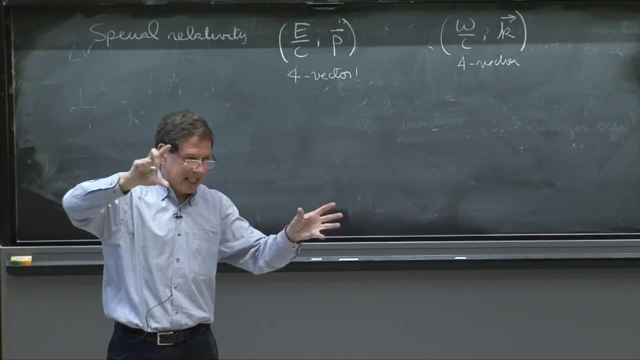 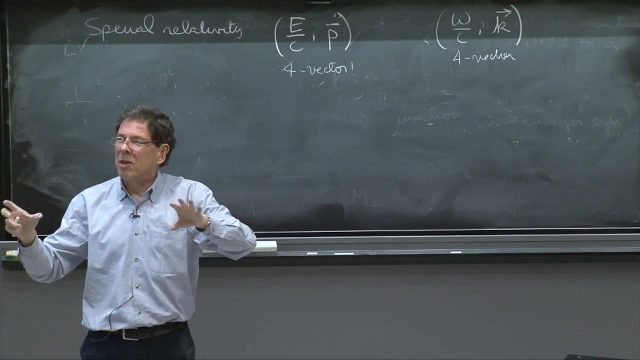 So this is also four vector in special relativity And therefore vector Vectors are things that transform nicely. So it makes sense to say that one four vector is equal to another four vector Because, if it's true, in one reference frame 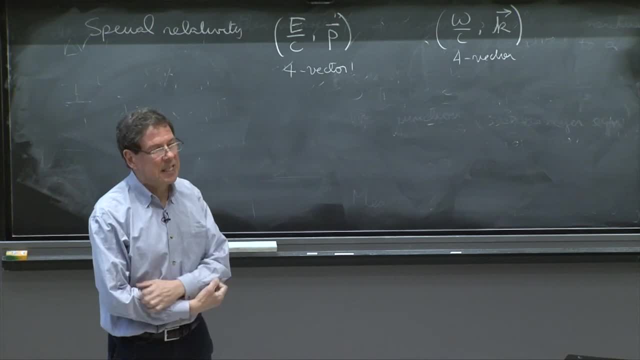 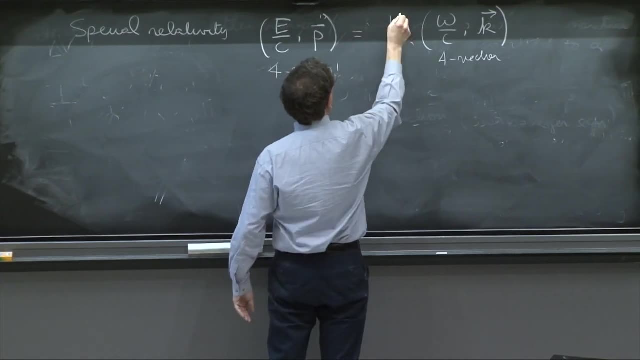 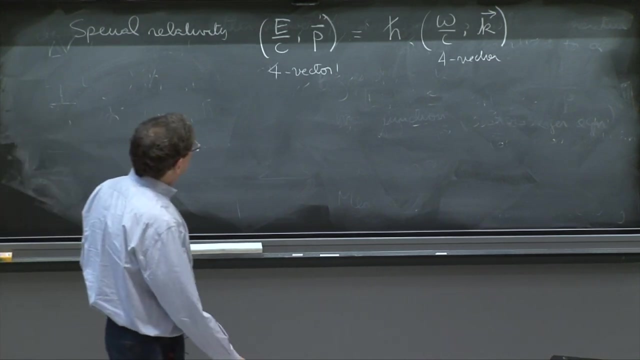 it will be true in every reference frame, So it's almost irresistible to make them equal, And de Broglie in some sense said: this is equal to h bar times that That's de Broglie. The Interesting thing is that this is true relativistically. 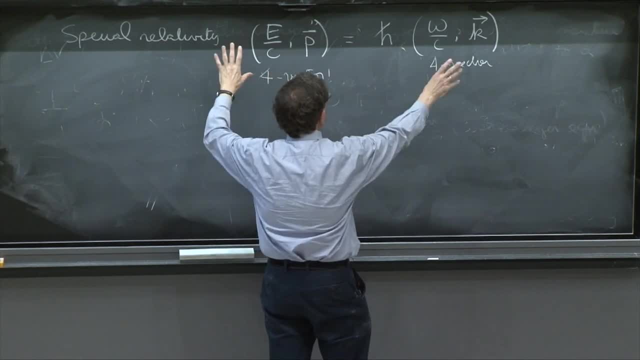 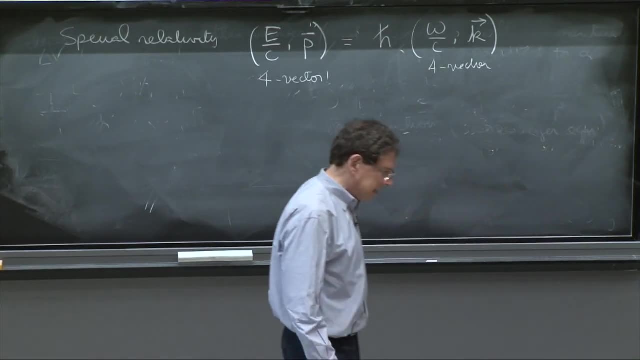 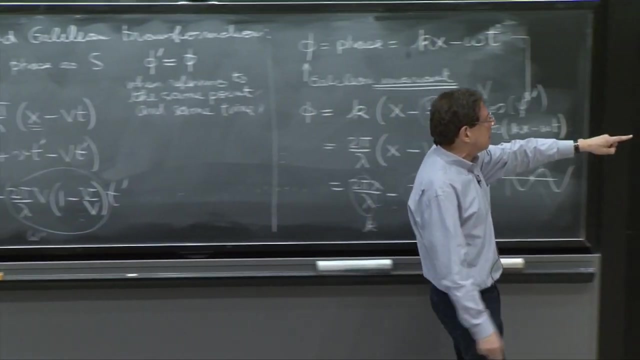 But actually non-relativistically you can make sense of this and set it equal, to be the same things, And the phase velocities, group velocities, all make sense. Certainly we've now said for matter particles that e is equal to h bar omega. 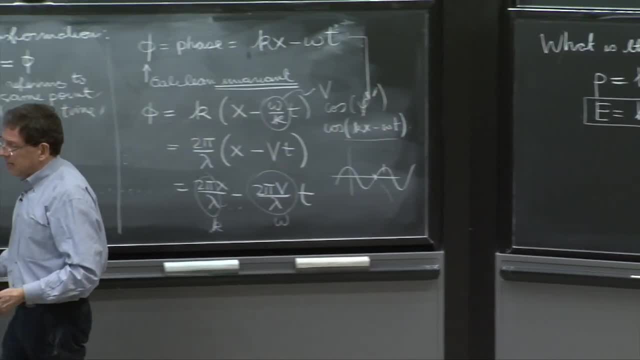 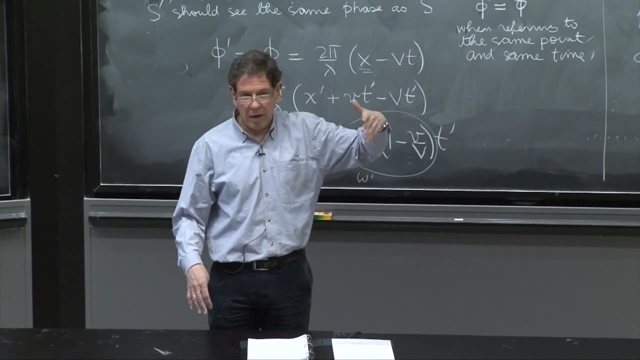 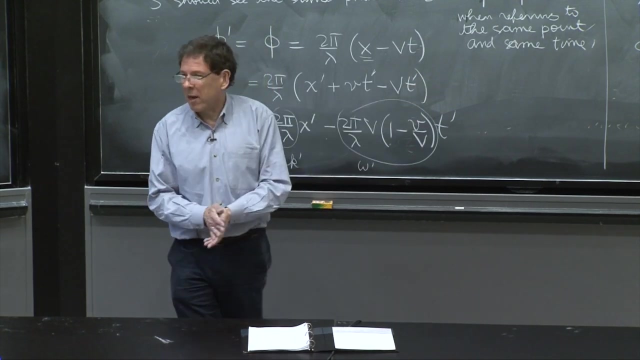 But another statement would be that, yes, indeed, Einstein said that That, for photons, e was equal to h bar omega or h nu, And therefore, yes, whatever happens for photons, happens for these matter waves, And so also, so this is another argument. 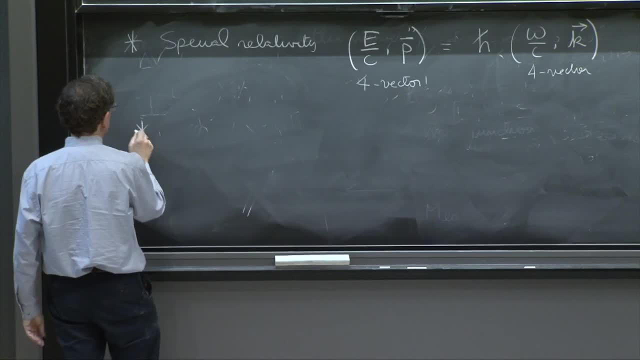 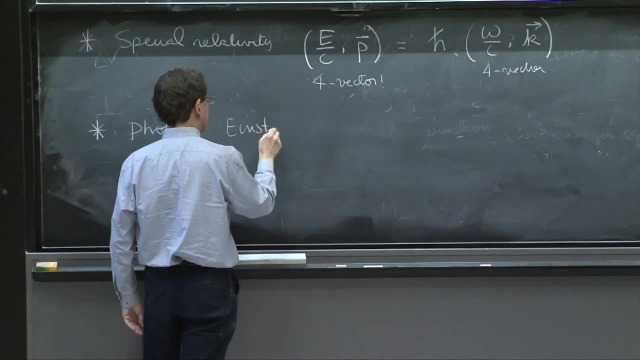 Group. velocities is one, Special relativity is another reason. And of course, photons, where Einstein said that e is equal to h nu, which is equal to h bar omega. 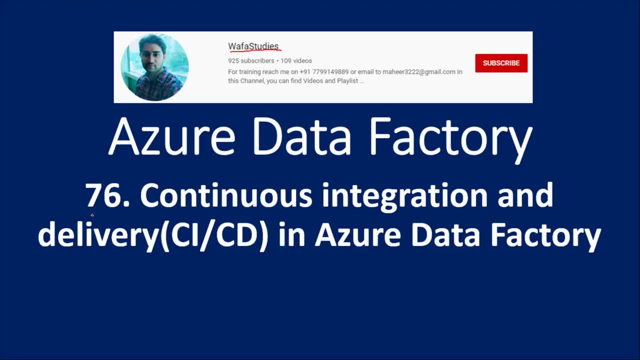 Hi friends, welcome to wafa studies. This is part 76 in azure data factory playlist. In this video we are going to discuss about continuous integration and delivery in azure data factory. So CI stands for continuous integration, CD stands for continuous delivery.